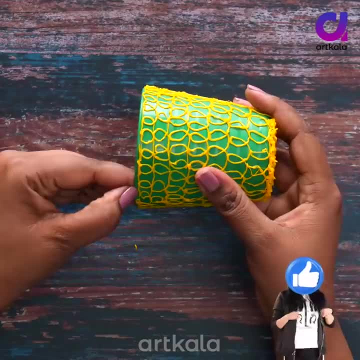 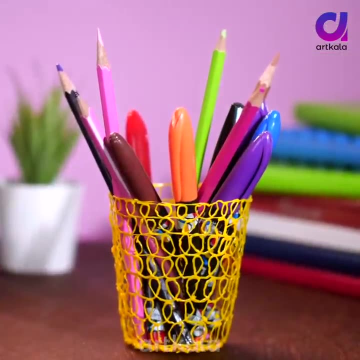 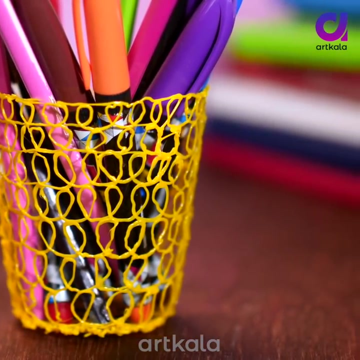 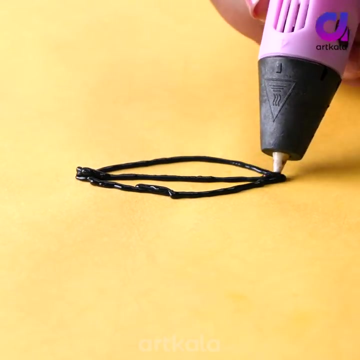 Like all the time, It still feels right. Stuck in an endless fight, Like every night, It still feels right. Even the words can't sing. I wanna change a thing, Cause without you Everything means nothing. You make me lose my mind. Like all the time, It still feels right. 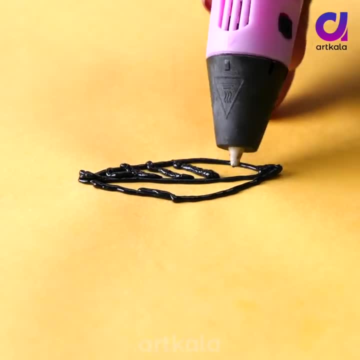 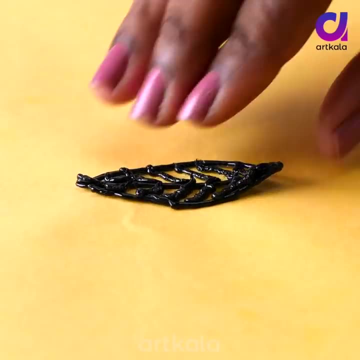 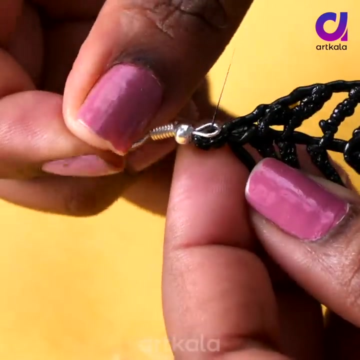 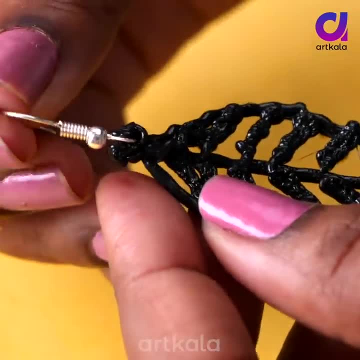 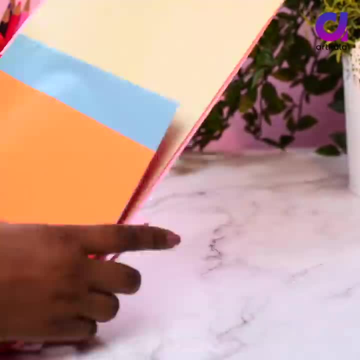 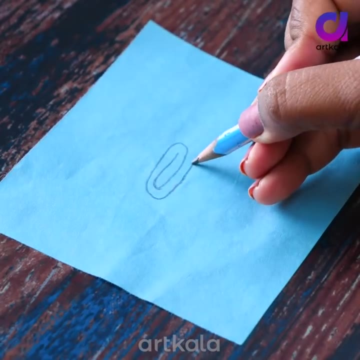 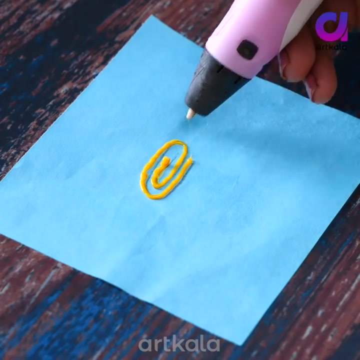 You think you know me, Say I'm as cold hearted as they come. You think I'm slowly Cutting my ties with you. That I'm done. Here's what you don't know: Feelings. they grow slow. I've just been caring for mine. Now I can feel it. 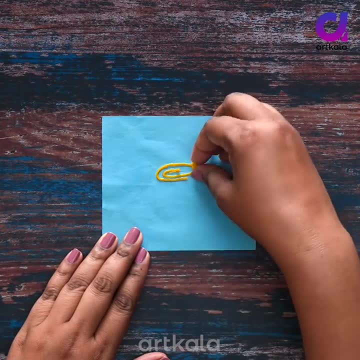 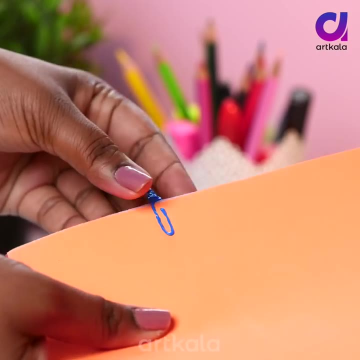 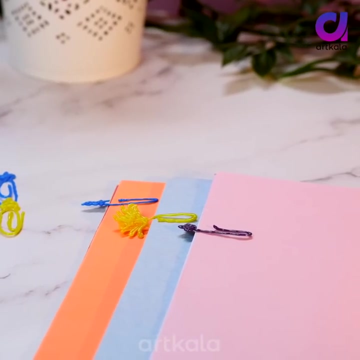 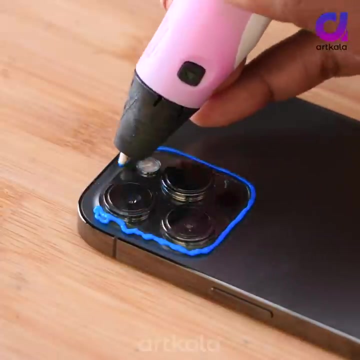 Now I believe it. Baby, tonight is the night. I'm gonna call you up In the name of love. Gonna call you up And tell you That I'm not giving up In the name of love. I'm not giving up Yet. I'm looking. In the name of love. 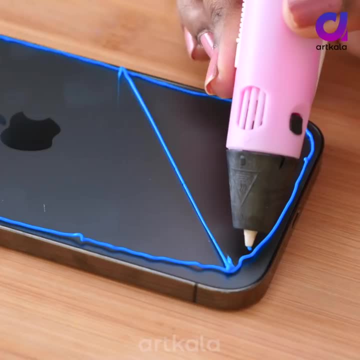 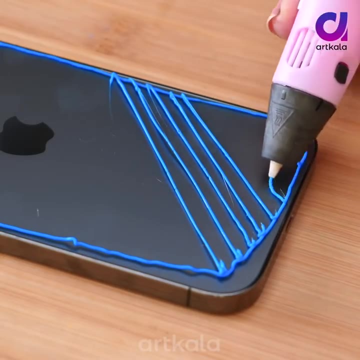 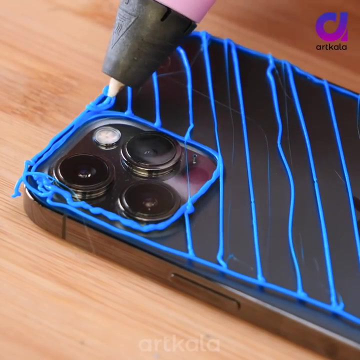 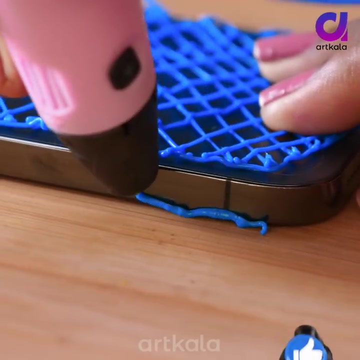 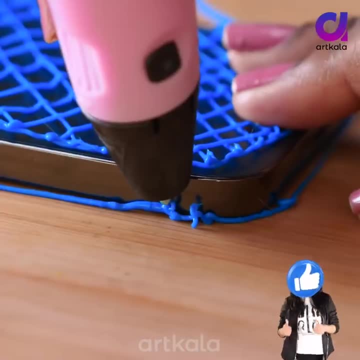 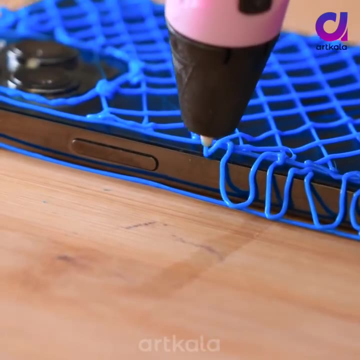 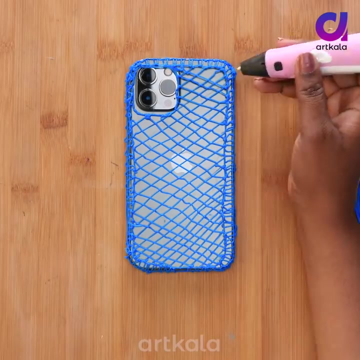 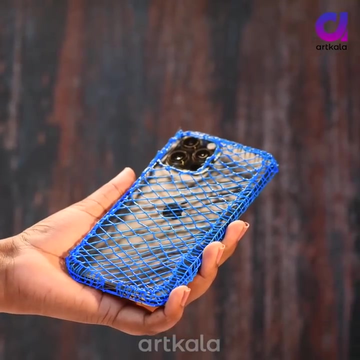 Here's what you don't know: Feelings. they grow slow. I've just been caring for mine. Now I can feel it, Now I believe it. Baby, tonight is the night. I'm gonna call you up In the name of love, Gonna call you up and tell you That I'm not giving up.